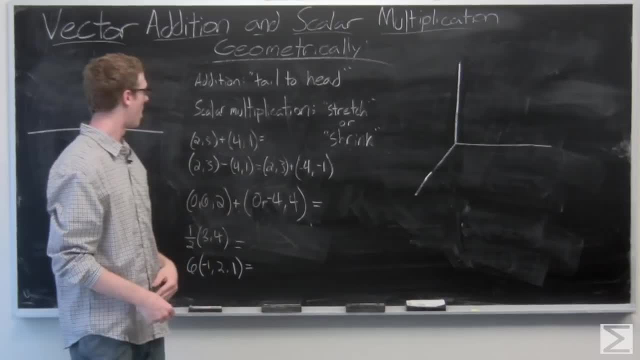 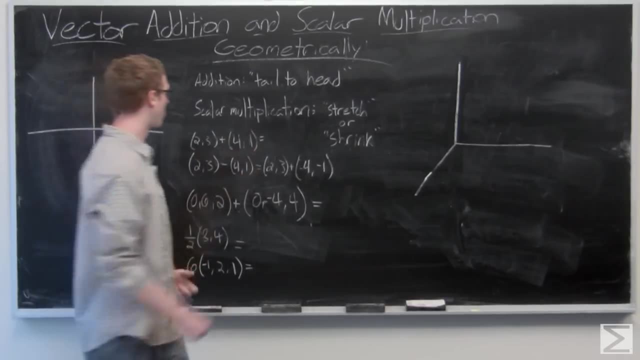 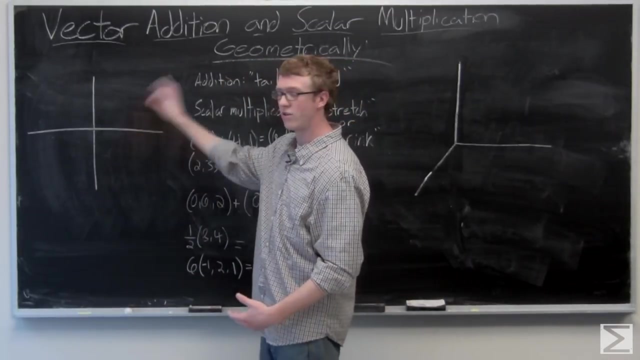 So we're just going to immediately check out an example of that. We have the vector 2 comma 3 plus the vector 4 comma 1, the resultant vector add component-wise 6 comma 4.. And we could just go ahead and draw a vector that is 6 comma 4, but let's take a look at 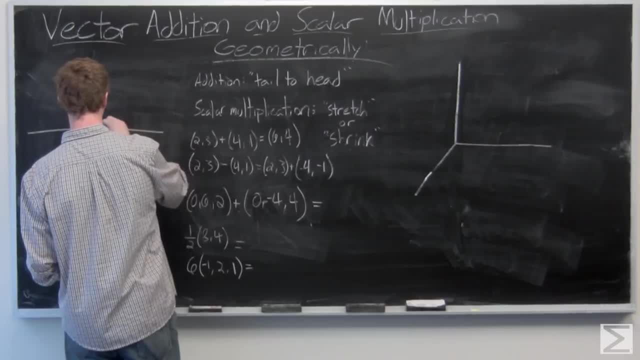 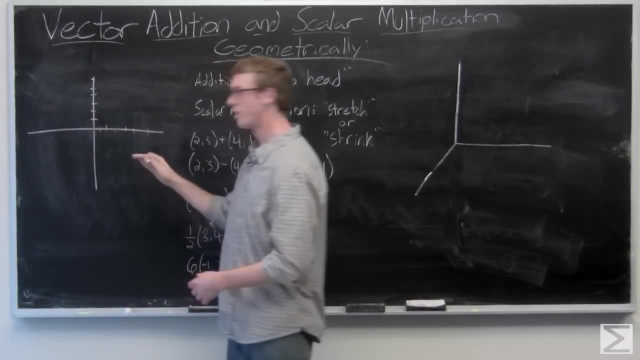 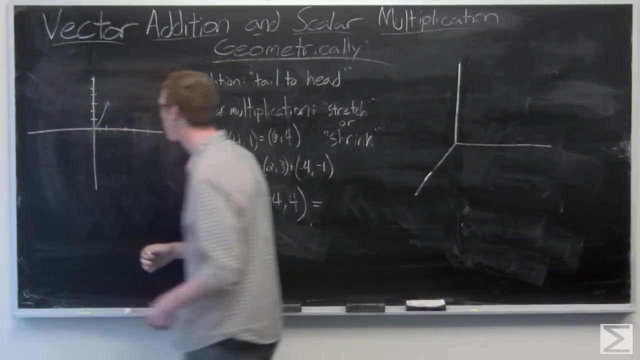 how we're going to get there. So this is our plane. We have a vector 2 comma 3,, 2 to the right, 3 up, And now we're adding the vector 4 comma 1.. So we're going to add the tail. 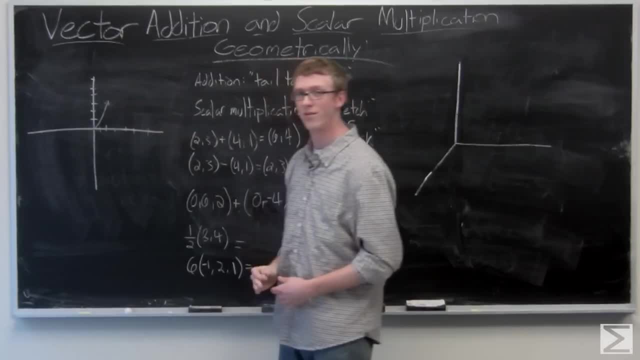 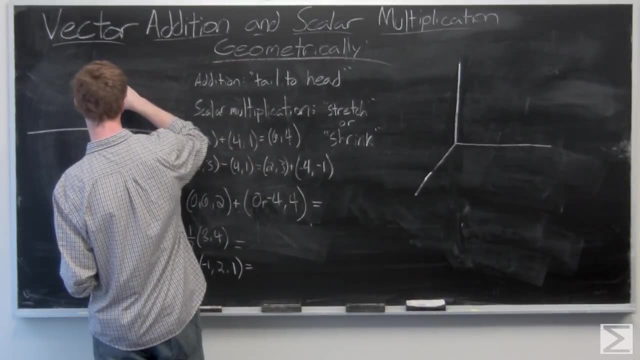 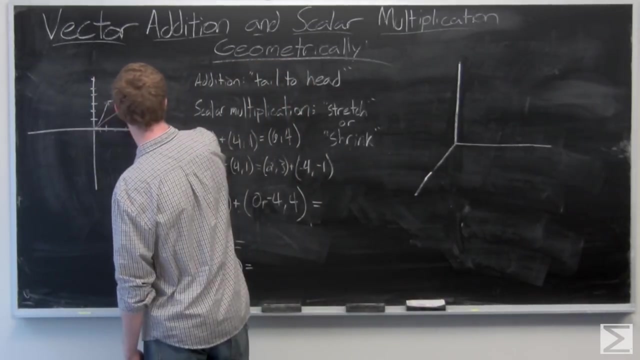 tail of the vector 4 comma 1 to the head of the vector 2 comma 3 to get the resultant 6 comma 4.. So our vector 6 comma 4 looks like this And we can see that we had addition to get there. 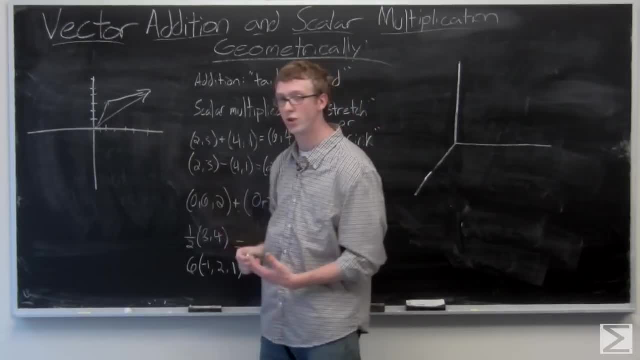 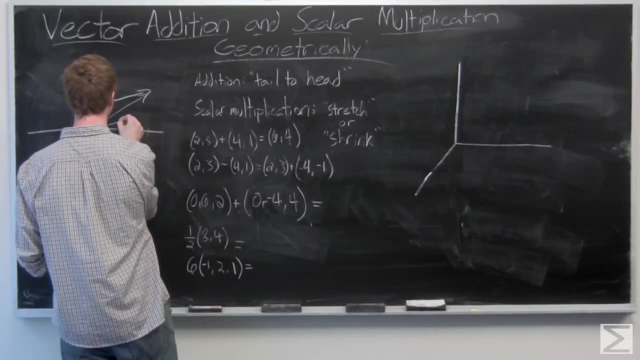 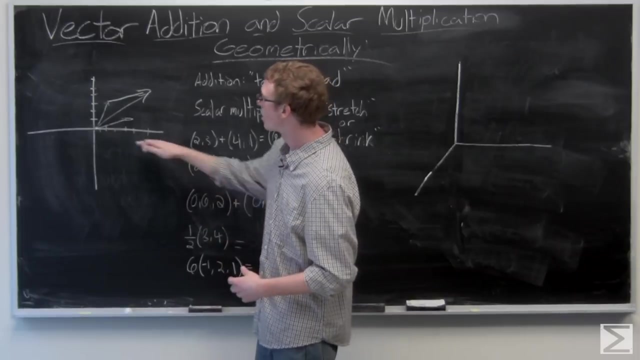 We could have also done it 4 comma 1 plus 2 comma 3.. We'll take a look at that Now. this is going to form a parallelogram. It's a little bit ugly in this situation because my coordinates are not exactly even, but you can get the picture. 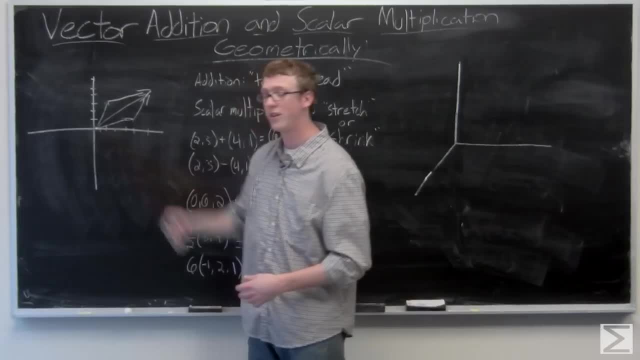 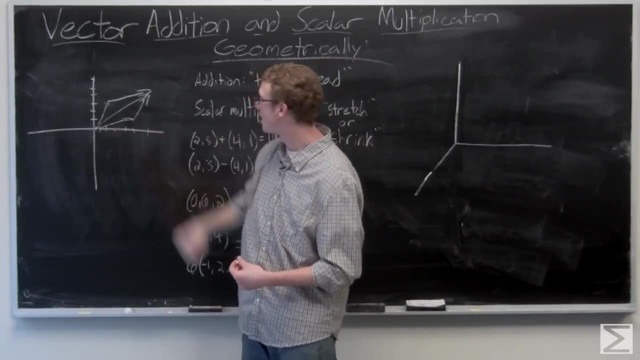 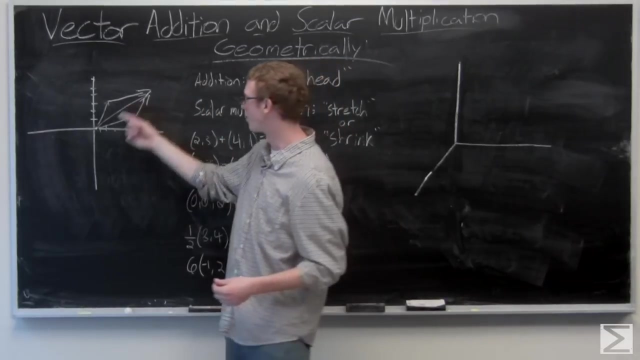 So you can either make a triangle or a parallelogram. The parallelogram method would be to have your tails connecting in the beginning, tail, tail here, And then you draw from there, from each head, the added vector, and you'll come to the conclusion that it's just the. 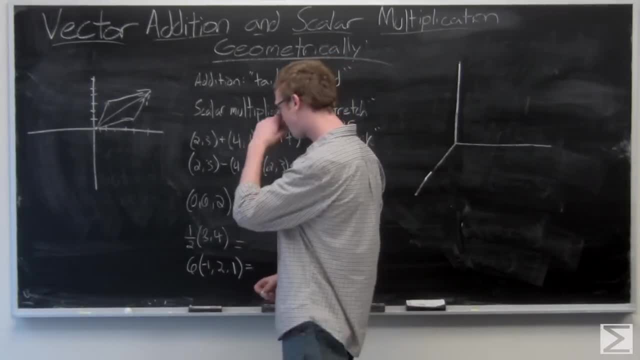 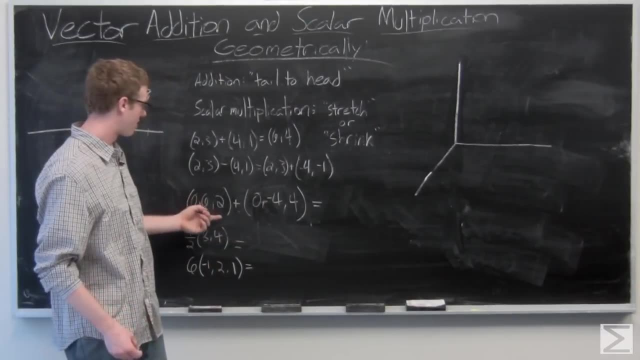 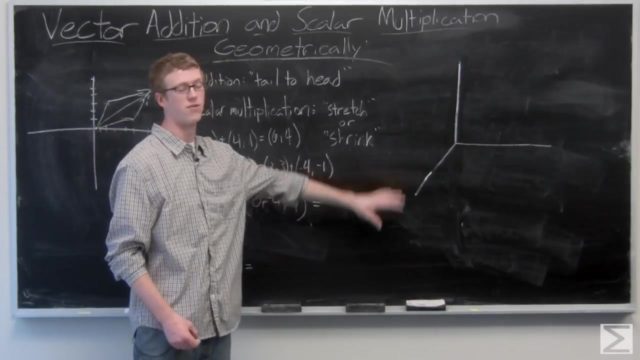 vector that we found with the triangle method. So now we can take a look in three space. we can take a look at some addition here. We have the vectors and I've made it pretty simple on myself so I don't have to draw anything confusing coming. 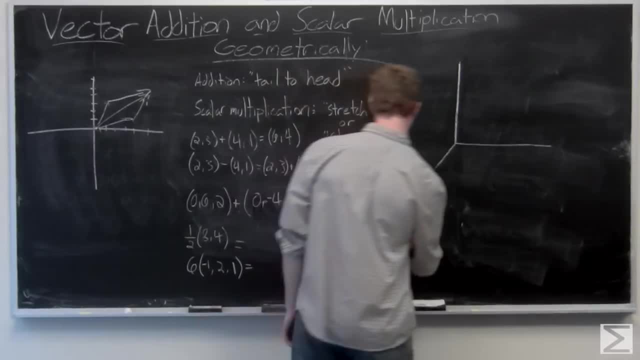 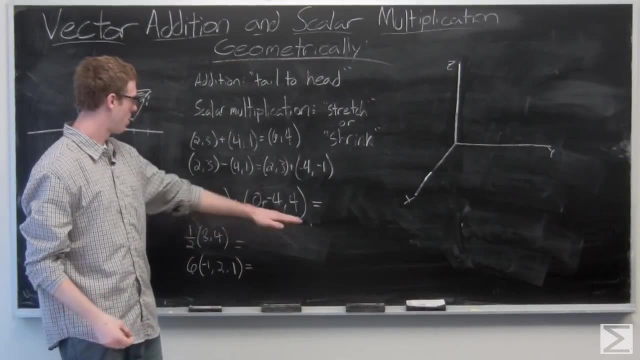 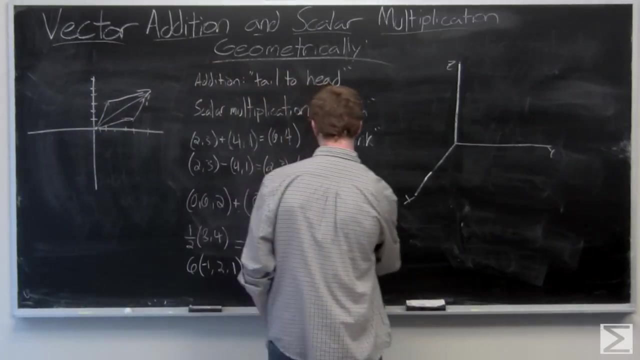 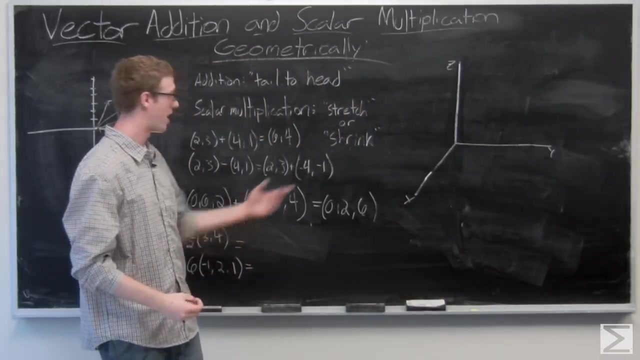 out of the board here, as this is our x-axis. So we have 0,, 6, 2 plus 0, negative 4, 4, add the vectors component-wise: 0,, 2, and 6.. So we'll take a look at this in three space. it's going to be a little bit more confusing. 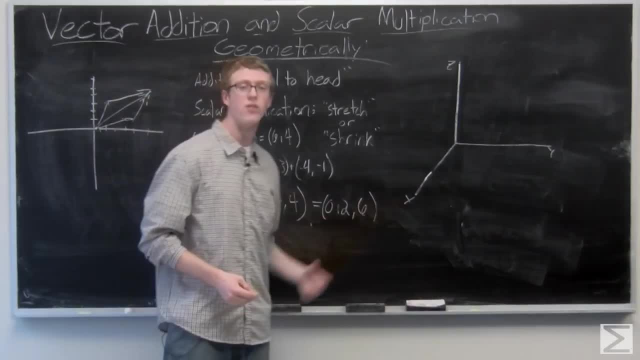 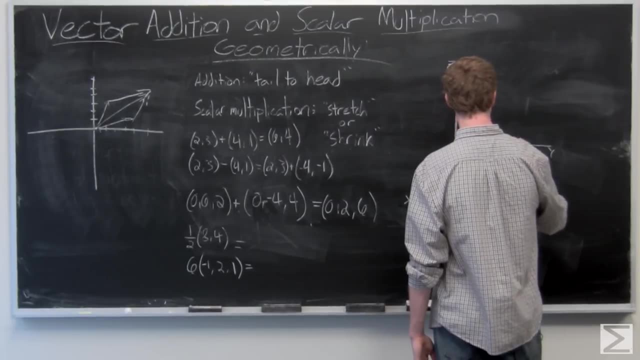 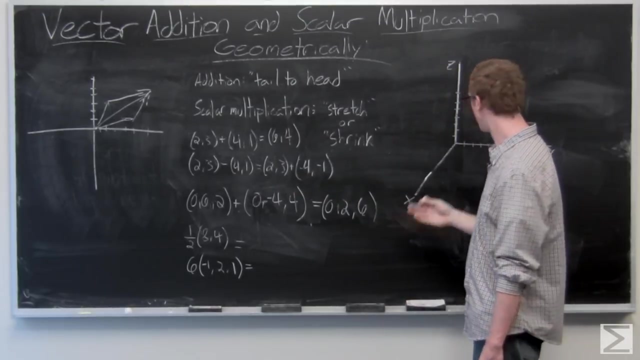 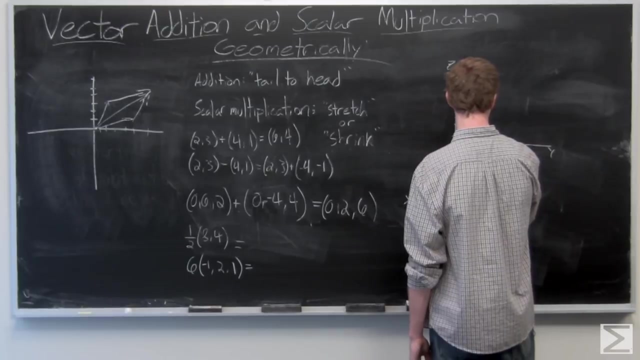 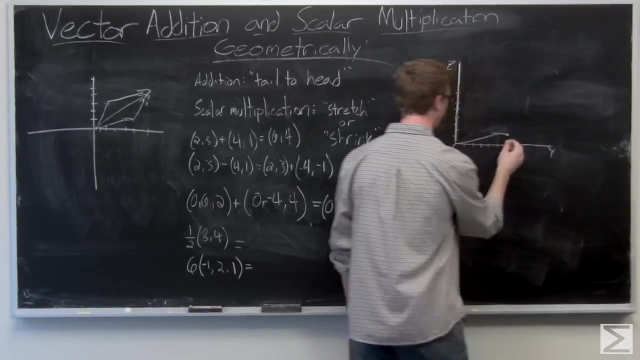 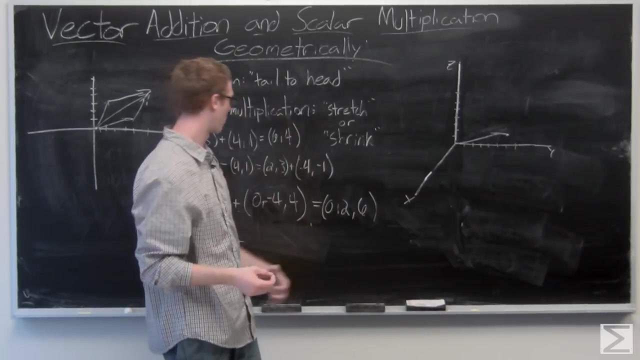 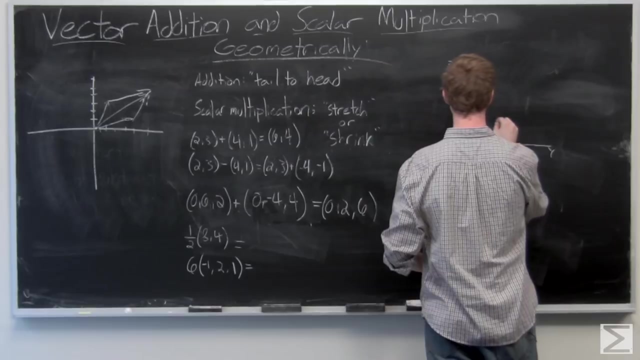 to draw when you have vectors that are coming out of the board. Better on the x-axis, So 6 in the y-direction, 2 in the z-direction And 0, negative 4,, 4, it's going to come back 4 and then up 4 more in the z direction. 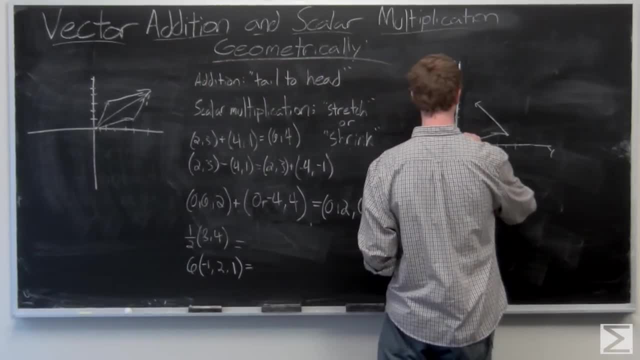 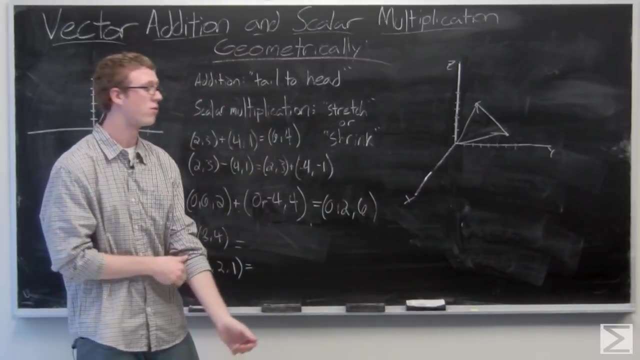 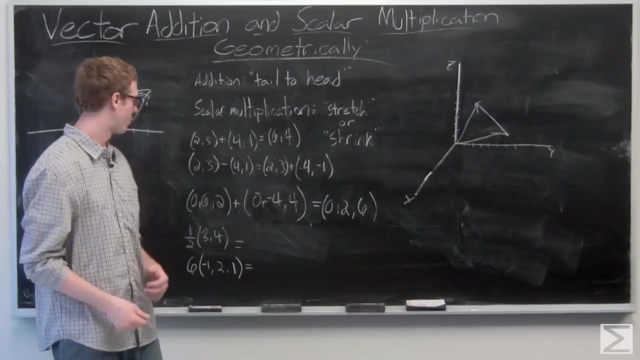 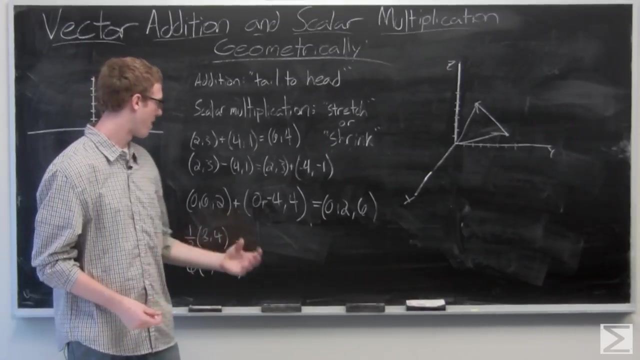 And the resultant vector is 0,, 2,, 6.. So again, adding component-wise and using this triangle rule to add your vectors- really great rule. Now we can take a look at the geometric interpretation of scalar multiplication. It's going to stretch or shrink your vector depending on if you're multiplying by a fractional. 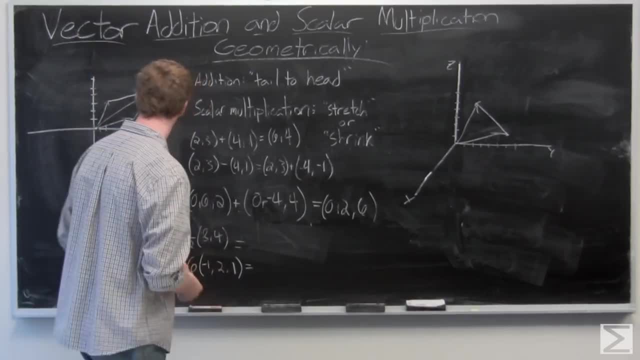 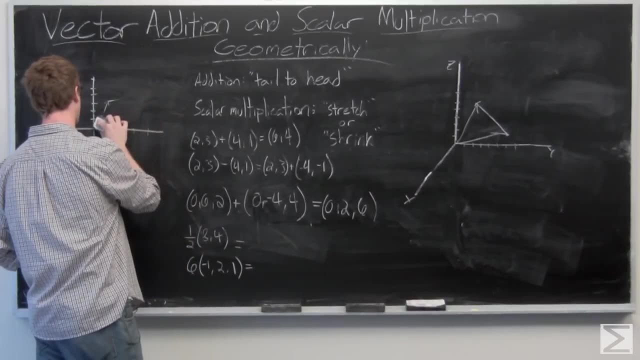 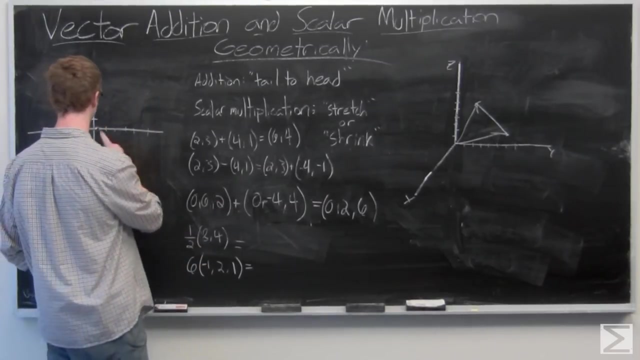 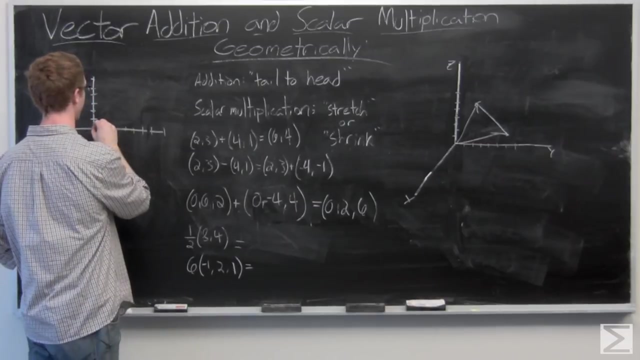 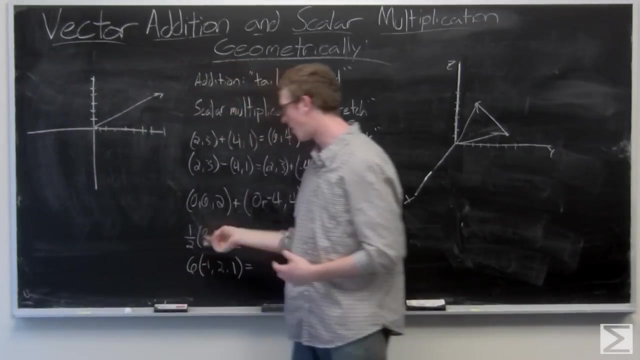 scalar, or if you're multiplying by a large scalar. So we're taking a look at half of 8 comma 4 in 2 space. So I'm just going to draw the vector 8 comma 4.. So here's your vector 8 comma 4.. 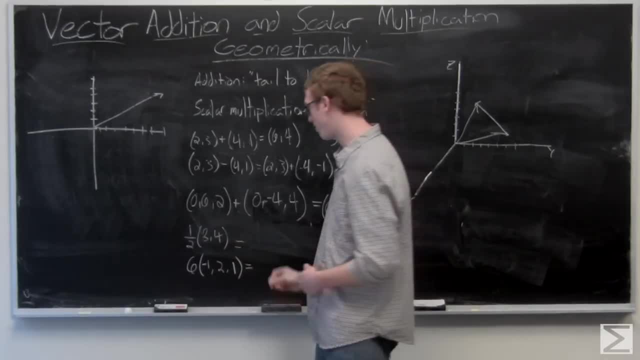 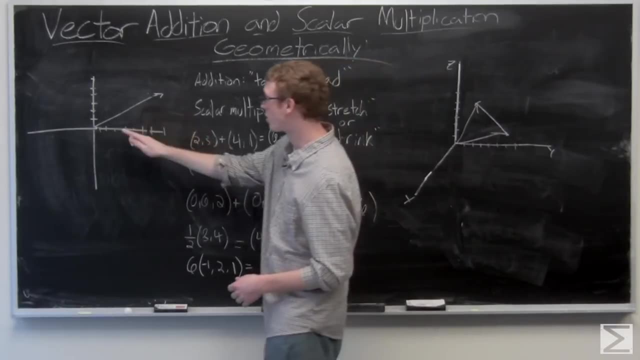 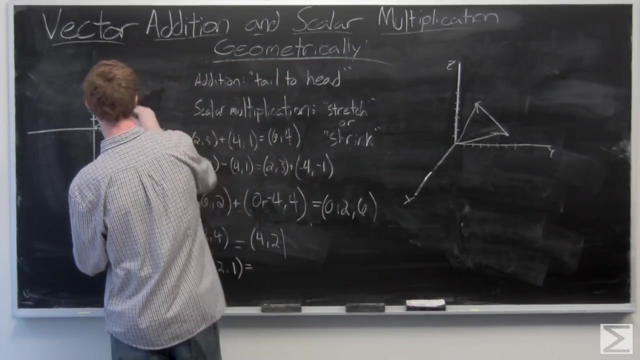 Now half of 8 comma 4, you just multiply each component by 1 half. Okay, So your resultant vector is 4, 2, and you're going to see a shrink from this long vector to a lot shorter vector 4 comma 2..